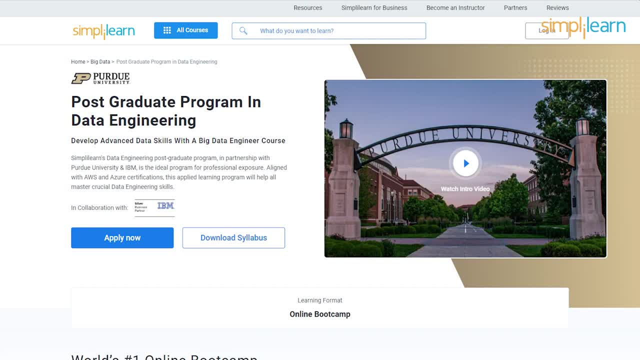 And in collaboration with leading industry experts. then search no more. Simply. Learn's postgraduate program in data engineering from Purdue University in collaboration with IBM, should be your right choice. For more details on this course, use the link in the description box below. 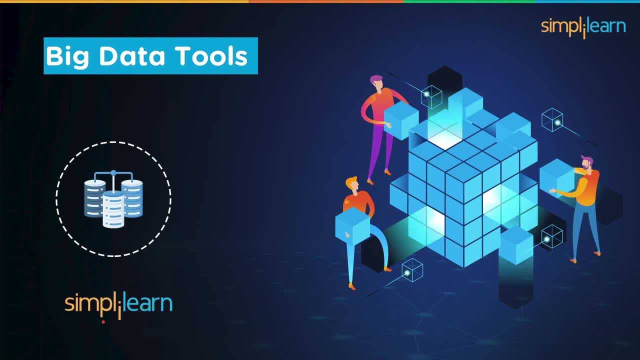 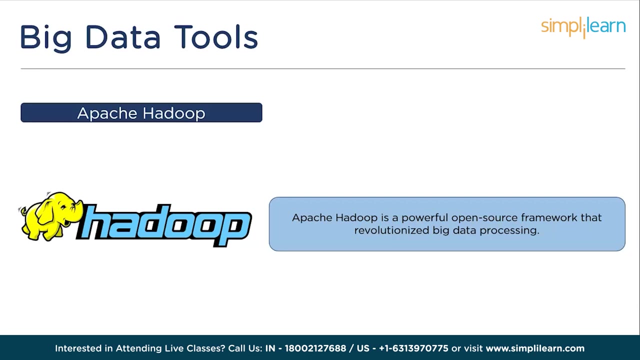 With that in mind, here's the list of the top 10 big data tools that are commonly used in the industry, which you need to know. We will get started with the first one, that is, Apache Hadoop. Apache Hadoop is a powerful open-source framework that revolutionized big data processing. 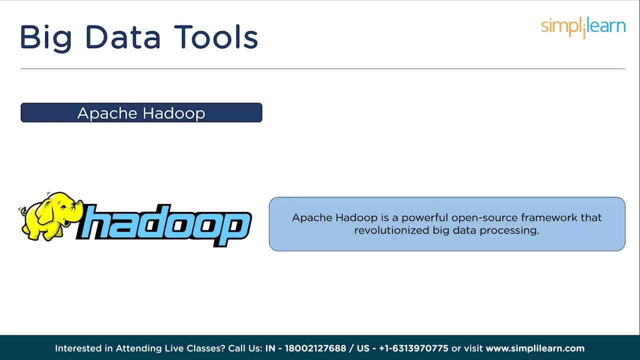 It enables the distributed processing of vast datasets across clusters of computers, providing scalability, fault tolerance and cost effectiveness. Hadoop's core components, Hadoop Distributed File System and MapReduce, allow data to be stored and processed in parallel, making it ideal for large-scale data analytics With Hadoop. 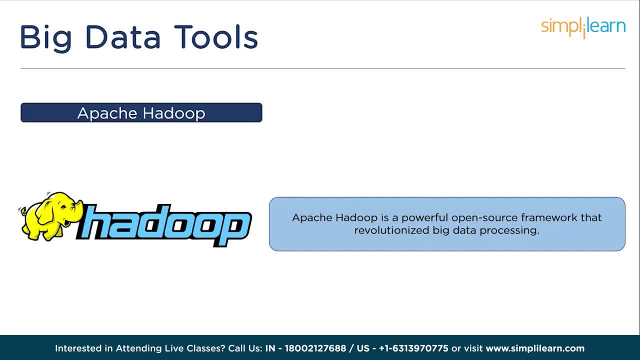 organizations can effortlessly store, manage and analyze structured and unstructured data, unlocking valuable insights. Its ecosystem of tools and technologies has made it a corner store in the big data landscape, empowering businesses to tackle complex data challenges and drive data-driven decision-making. The second one in the list is Apache Spark. 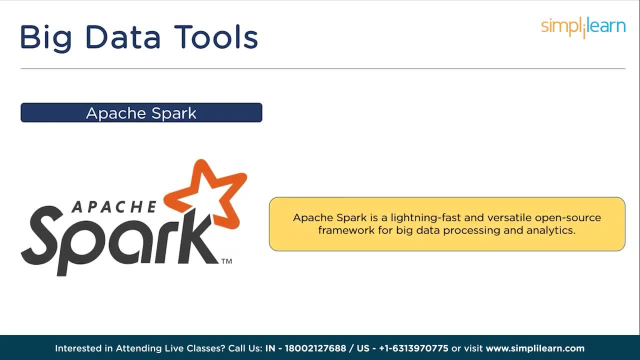 Apache Spark is a lightning-fast and versatile open-source framework for big data processing and analytics. It provides an in-memory computing engine that accelerates data processing, making it ideal for real-time analytics, machine learning and iterative algorithms. Spark's rich set of APIs supports various programming languages. 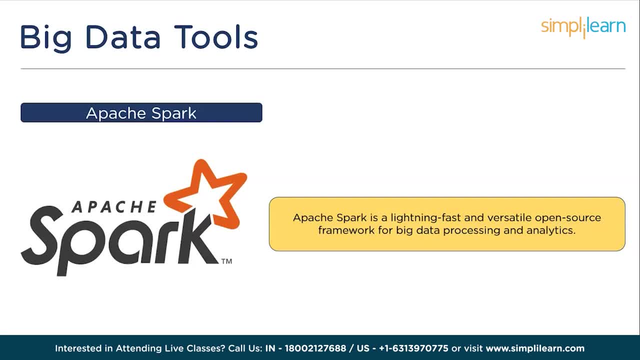 allowing developers to work with ease. It offers modules for streaming, SQL, machine learning and graph processing, making it a comprehensive tool for diverse data tasks. With its ability to handle large-scale data processing, Spark has become a popular choice for organizations looking to extract valuable insights from their big data. 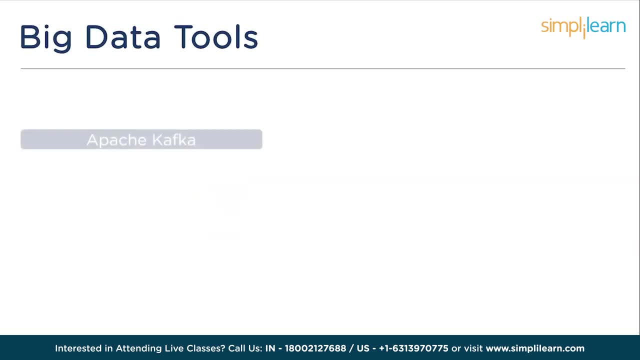 quickly and efficiently. The third one on the list is Apache Kafka. Apache Kafka is the third-largest data processing platform in the world. It has the highest capacity, the largest users, the largest data sources and the most complex data collection. It is a single-use platform for all types of data processing and analytics. The third one on the list is Apache Kafka. 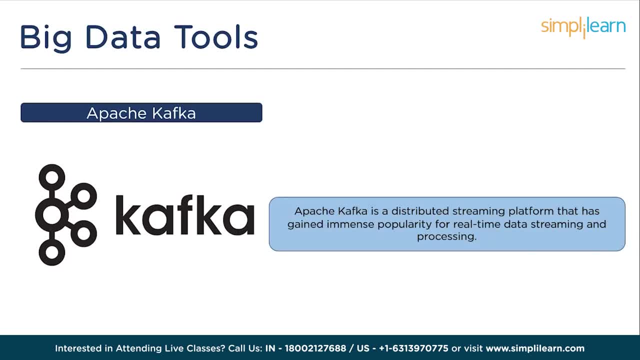 Apache Kafka is a distributed streaming platform that has gained immense popularity for real-time data streaming and processing. It provides a fault-tolerant, scalable and high-throughput messaging system that enables the building of real-time data pipelines and applications. Kafka's unique design allows it to handle high volumes of data and seamlessly integrate. 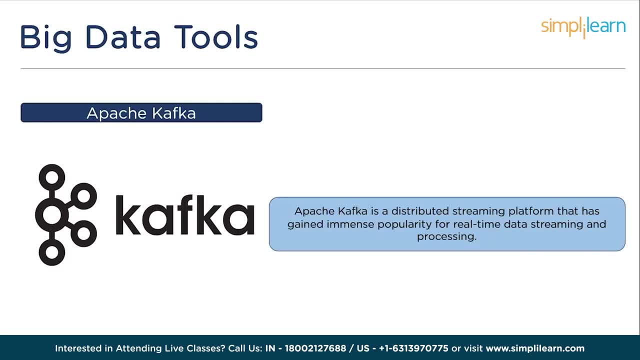 with various data sources and sinks. It follows a publish-subscribe model where producers publish messages to topics and consumers subscribe to those topics to receive and process the messages in real-time. Kafka's versatility and reliability make it a crucial tool for data ingestion stream. 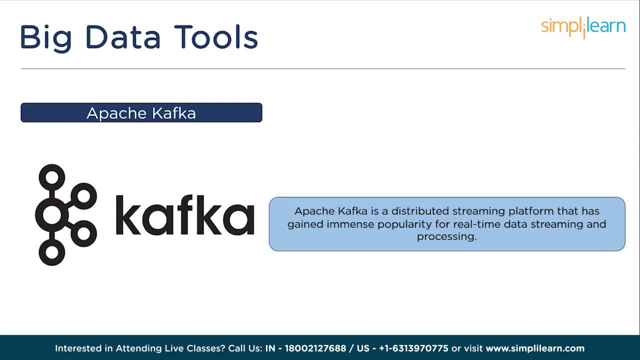 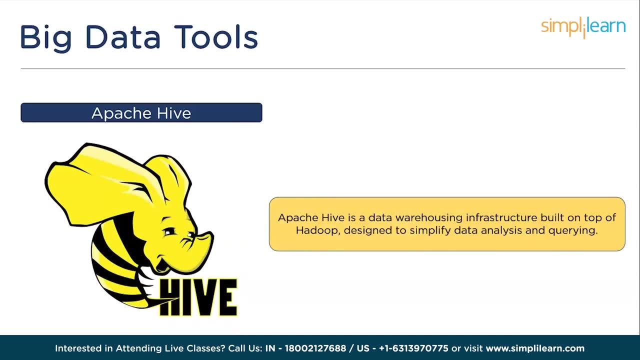 processing and event-driven architectures in modern data-driven organizations. Fourth one on the list is Apache Hype. Apache Hype is a data warehousing infrastructure built on top of Hadoop, designed to simplify data analysis and query. It provides a SQL-like interface allowing users to write queries. 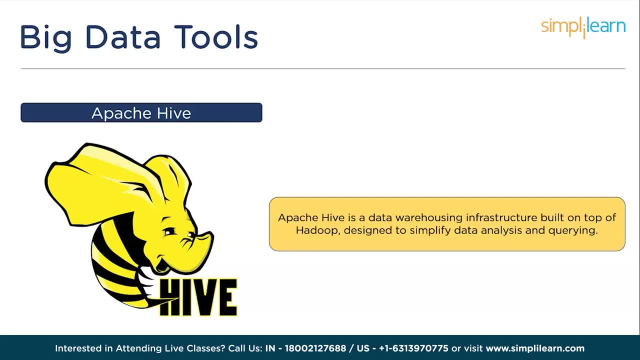 Hive translates queries into MapReduce jobs, making it easy for analysts and data scientists to work with big data without writing complex MapReduce code. It supports various data formats, partitioning and schema evolution. Hive is particularly useful for batch processing and ad-hoc queries, enabling users to extract. 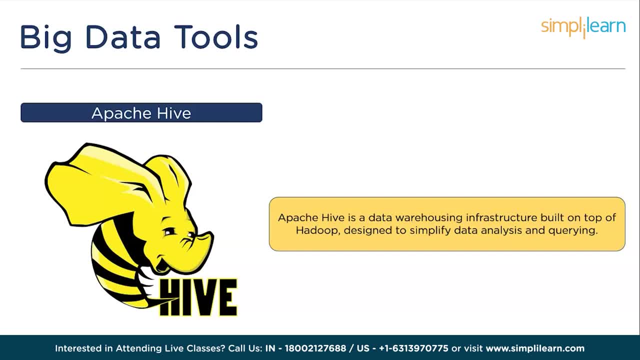 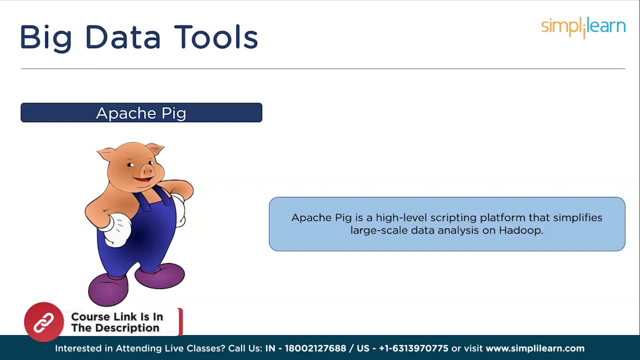 insights and perform data exploration efficiently. It plays a crucial role in enabling data-driven data-generation making in organizations and companies. Fifth one on the list is Apache Pig. Apache Pig is a high-level scripting platform that simplifies large-scale data analysis on Hadoop. 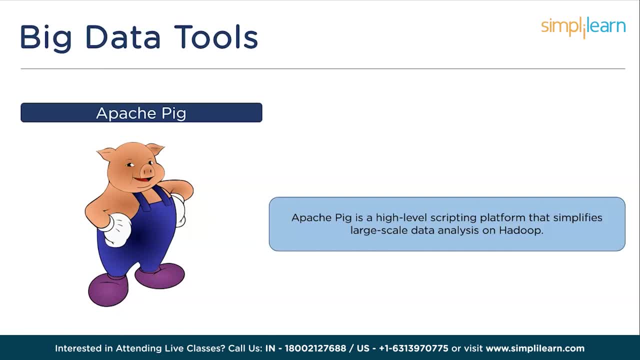 It provides a programming language called Pig Latin, which abstracts the complexities of writing MapReduce jobs. With Pig, users can express data transformations and analytical tasks using a simple and intuitive scripting language, making it accessible to data analysts and scientists. Pig automatically optimizes and executes these tasks in parallel, enabling efficient 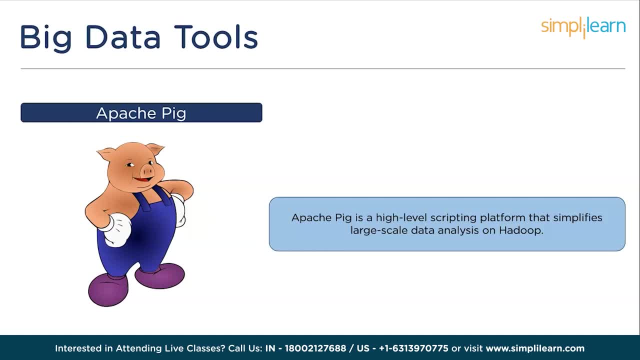 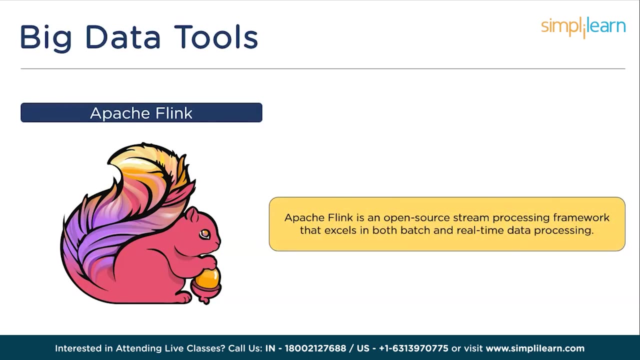 processing of large datasets. It supports a wide range of data types and offers a rich set of operators for data manipulation. Apache Pig is a valuable tool for batch processing and iterative analytics in big data environments. Sixth one on the list is Apache Flink. 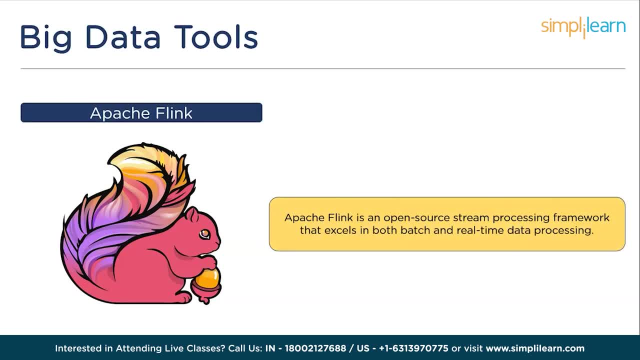 Apache Flink is an open-source stream processing framework that excels in both batch and real-time data processing. With its fault-tolerant and scalable performance, it's a great tool for batch processing and real-time data processing architecture. Flink enables the processing of continuous streams of data. 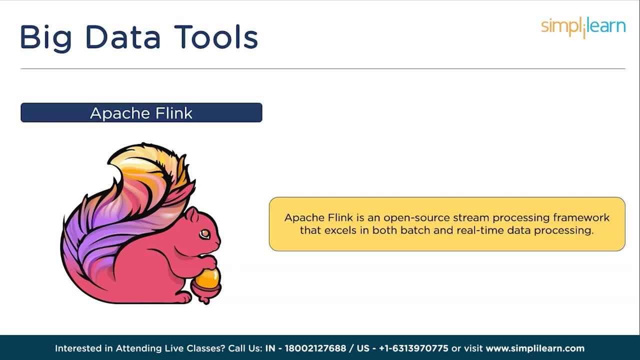 with low latency. It supports event time processing and stateful computations, making it suitable for complex analytics and machine learning tasks. Flink's flexibility allows users to build data pipelines and applications that seamlessly integrate batch and stream processing. Flink's flexibility allows users to build data pipelines and applications that seamlessly integrate. 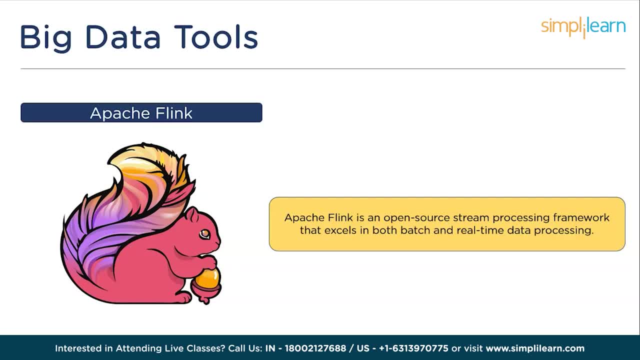 batch and streaming data. Its robust set of features including windowing, fault tolerance and exactly once processing positions. Its robust set of features, including windowing, fault tolerance and exactly once processing positions. Flink has a powerful tool for handling real-time data processing requirements. 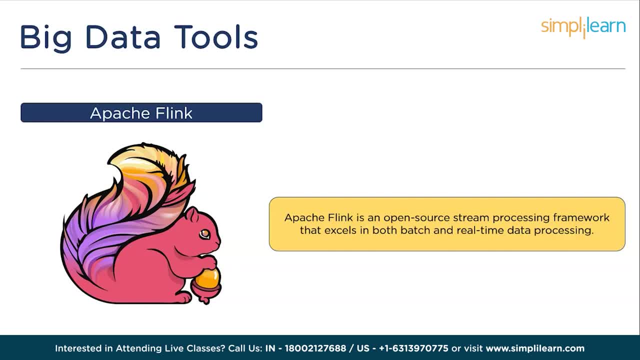 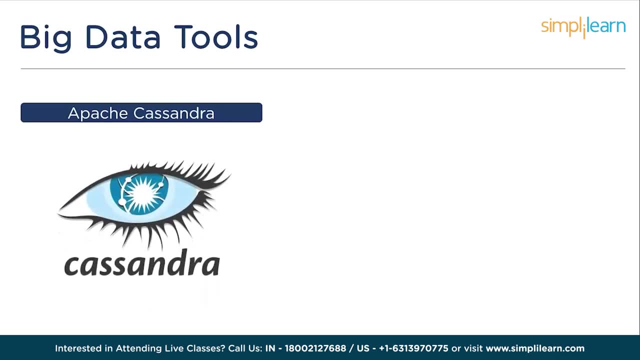 and enabling advanced analytics on streaming data. Seventh one on the list is Apache Cassandra. Apache Cassandra is a highly scalable and distributed NoSQL database designed to support the use of data processing tools and to handle massive amounts of data across multiple commodity servers. It offers. 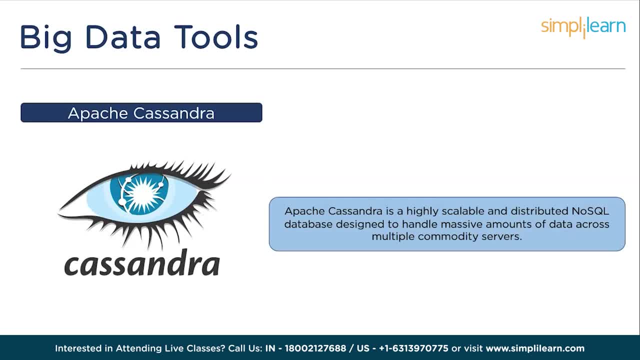 high availability, fault tolerance and tunable consistency levels, making it suitable for use cases that require high performance and scalability. Cassandra's decentralized architecture and peer-to-peer application ensures data durability and seamless scalability as data volumes grow. It provides a flexible data model and supports fast read and write operations, making it ideal for 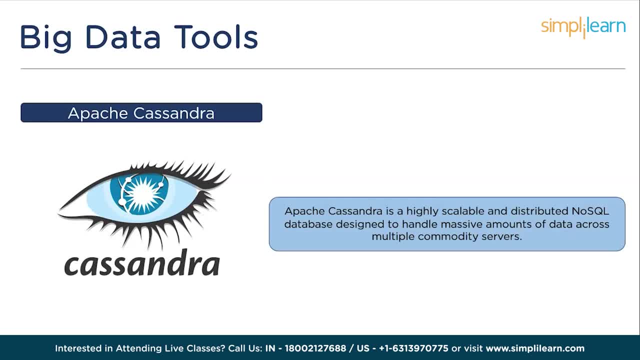 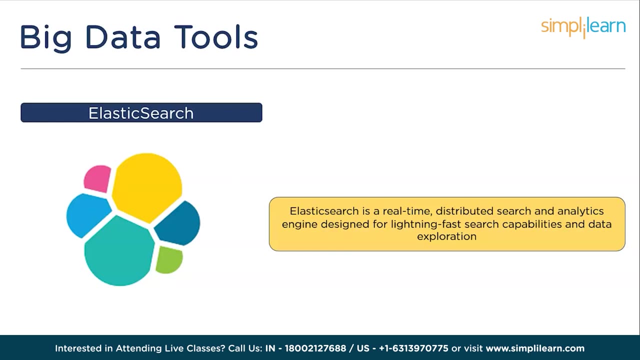 real-time applications, Time-series data and large-scale data ingestion. with its robust features, Cassandra empowers organizations to handle big data workloads with ease and reliability. Eighth one on the list is Elasticsearch. Elasticsearch is a real-time distributed search and analytics engine designed for lightning-fast search capabilities and 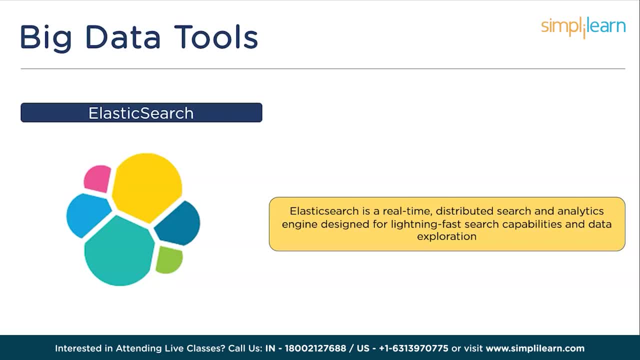 data exploration. It allows users to store, search and analyze large volumes of data in near real-time, making it a powerful tool for various use cases like log analysis, monitoring and full-text search. Elasticsearch is built on top of the Luenz search library. 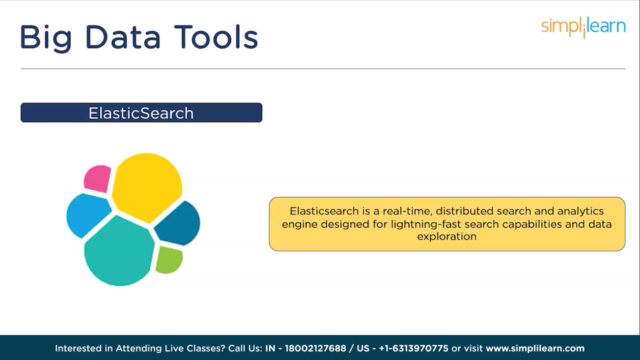 and provides a scalable distributed architecture that can handle high throughput workloads. It supports advanced search features, aggregations and geo-search capabilities, making it an essential tool for businesses that require fast and accurate data retrieval and analysis. Now ninth one on the list, which is Apache Storm. Apache Storm is a distributed real-time. computation system designed for processing, data processing and data processing. It is designed for processing, data processing and data processing. It is designed for processing, data processing and data processing. It is designed for processing, data processing and data processing. 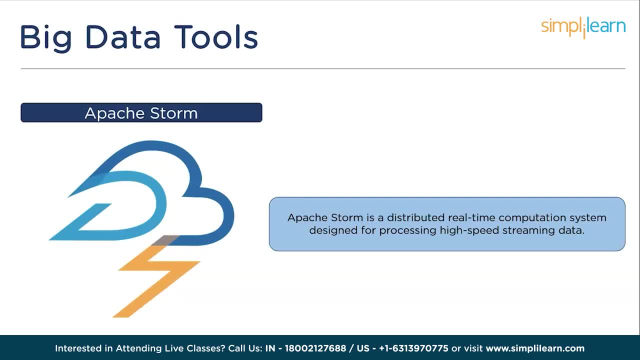 Next we have High-speed streaming data. It provides a scalable and fault-altered platform for real-time analytics, making it ideal for applications that require low latency in processing. Storm's architecture enables the parallel execution of data processing tasks, allowing for seamless scalability and high throughput. It supports various programming. 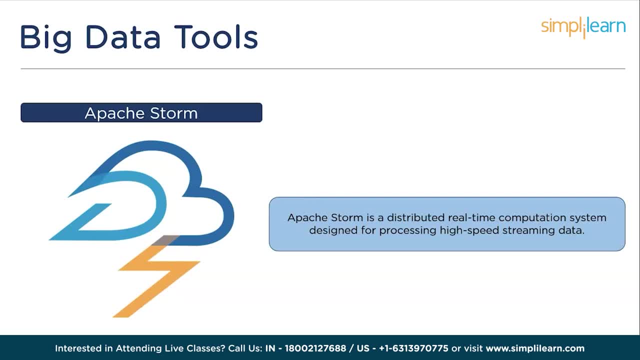 languages and provides reliable message processing with guaranteed data delivery, stress-financed telecommunications and social media. Real-time data processing is crucial for detecting fraud, monitoring trends and making it immediate business decisions. with storm organizations can harness the power of real-time data and respond swiftly to changing conditions. 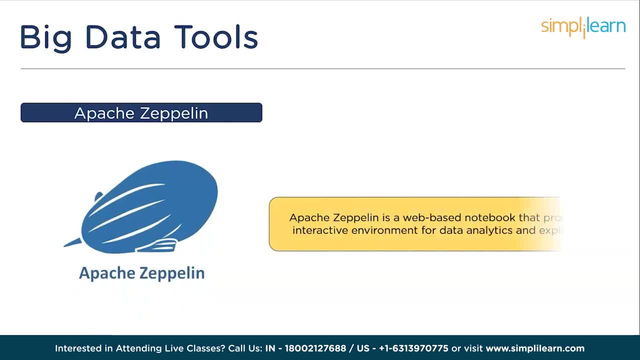 and finally, we have apache zeppelin. apache zeppelin is a web-based notebook that provides an interactive environment for data analytics and exploration. it supports multiple programming languages, including python, scalar and sql, allowing users to write and execute code snippets in collaborative and intuitive manner. zeppelin facilitates data visualization by integrating 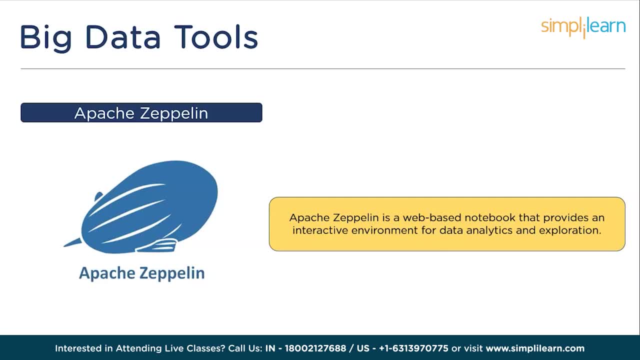 with popular visualization libraries and provides real-time visualizations for quick insights. it enables the creation of interactive documents, known as notebooks, which combine live code visualizations and narrative text. with its flexible and user-friendly interface, zeppelin empowers data scientists and analysts to explore, analyze and share their findings efficiently, making it valuable tool in their big data ecosystem. 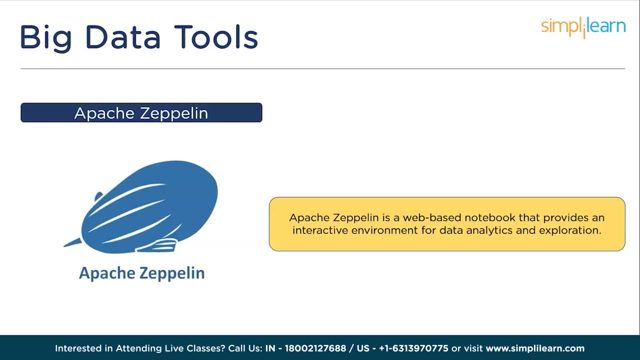 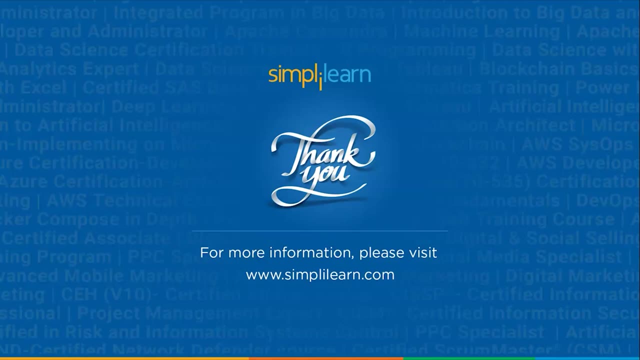 these are just a few examples of the top big data tools available in the industry. each tool has its own strength and use cases, so it's important to consider your specific requirements when choosing the right tool for your big data project. with that, we have reached the end of this session on the top big data tools. should you have any queries regarding any of the 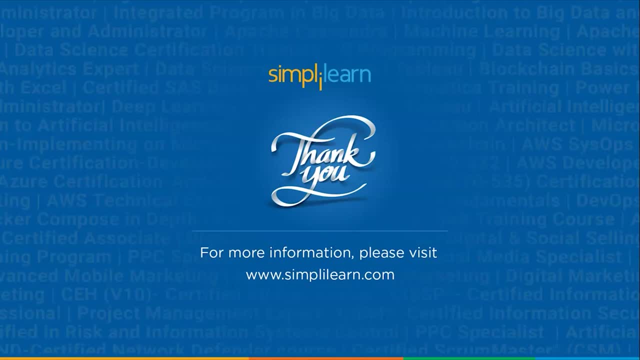 topics discussed in this session, then please feel free to let us know in the comment section below, and our team of experts will be more than happy to assist you with all your queries and concerns. and until next time, thank you for watching, and stay tuned for more from simply gone: staying ahead in your career.